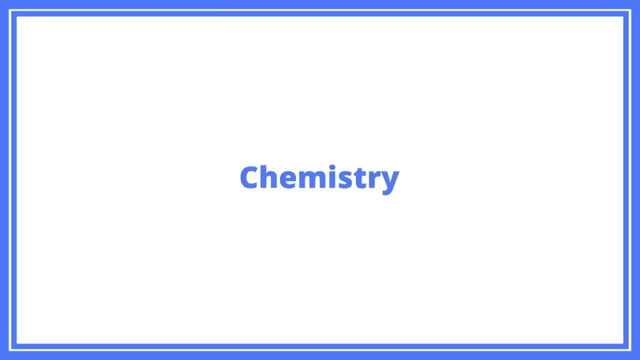 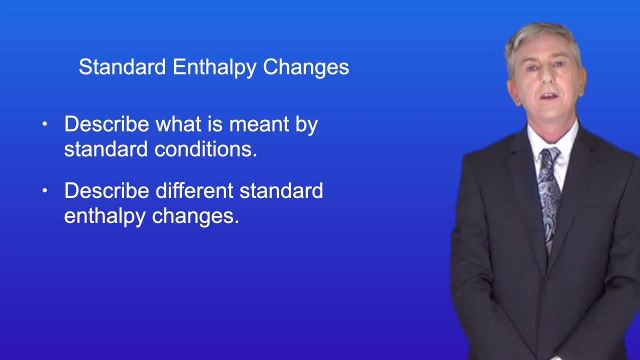 Hi, welcome back to Free Science Lessons. By the end of this video you should be able to describe what's meant by standard conditions. You should then be able to describe different standard enthalpy changes. In the last video we saw that enthalpy tells us the heat energy. 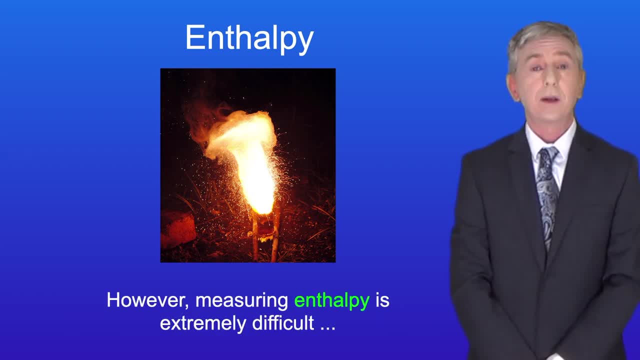 in a chemical system, However, measuring enthalpy is extremely difficult, so instead we determine enthalpy change. Now, one key idea you need to understand is that we always determine enthalpy changes under standard conditions. We refer to these as standard enthalpy changes. 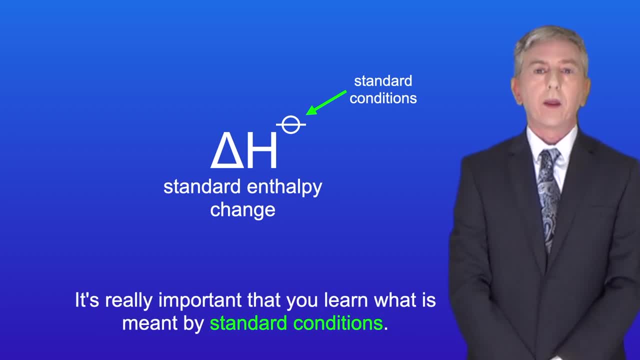 and they have this symbol. It's really important that you learn what's meant by standard conditions. Firstly, standard temperature is 298 Kelvin, which is 25 degrees Celsius. Standard pressure is 100 kilopascals. Standard concentration is one mole per decimetre cubed for chemicals in solution. And finally, all chemicals must. 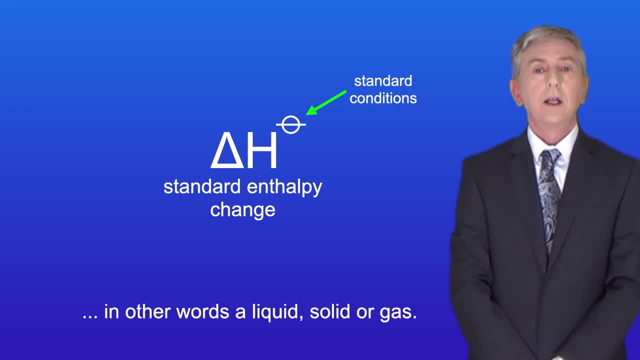 be in their standard states under standard conditions, In other words, a liquid, solid or gas. The unit for standard enthalpy change is kilojoules per mole. OK, now there are four different standard enthalpy changes that you need to understand. 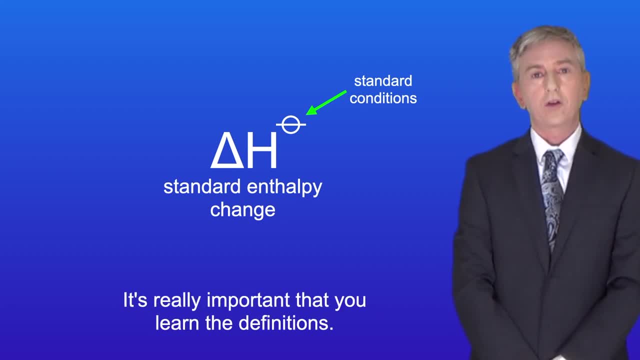 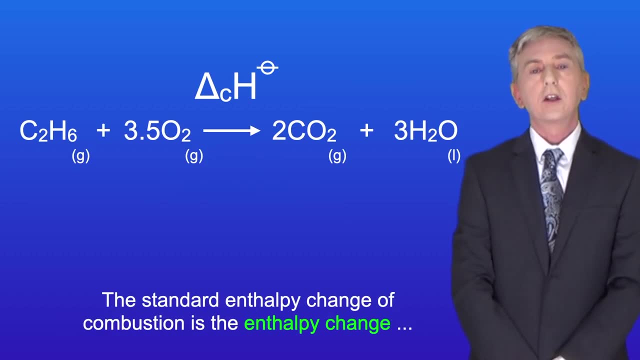 I'm going to take you through these in this video and it's really important that you learn the definitions. The first is called standard enthalpy changes. The standard enthalpy change of combustion is the enthalpy change when one mole of a 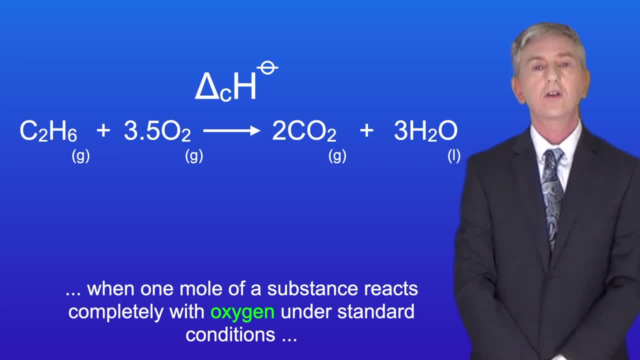 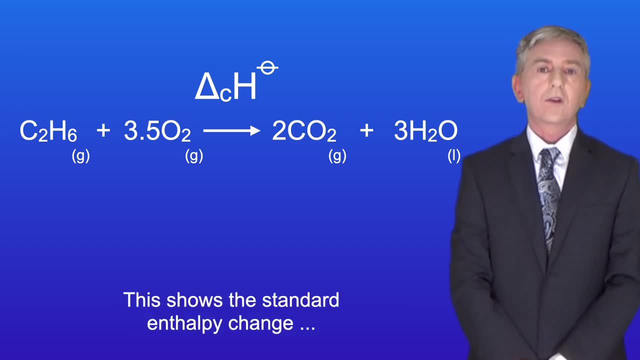 substance reacts completely with oxygen under standard conditions and all of the chemicals are in their standard states. I'm showing you an example here. This shows the standard enthalpy change for the complete combustion of the hydrocarbon ethane. Now there are 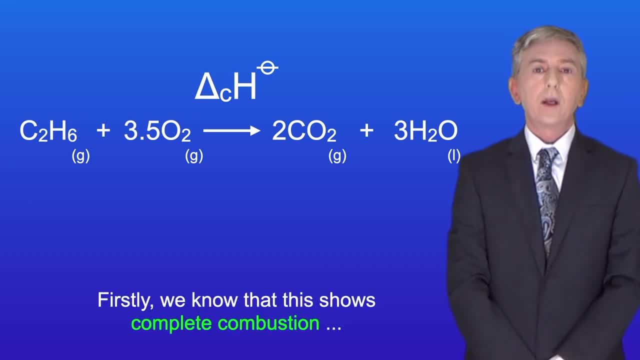 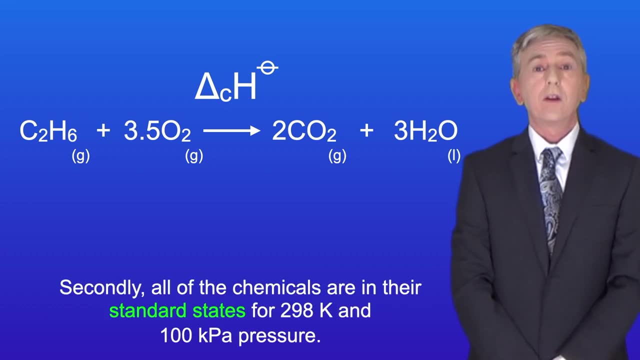 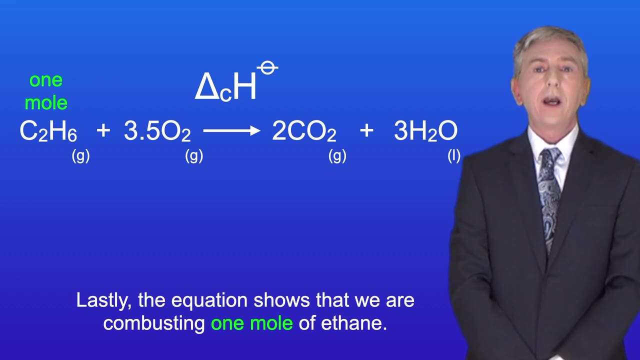 several points about this that you need to consider. Firstly, we know that this shows complete combustion, as we've made carbon dioxide. Secondly, all of the chemicals are in their standard states for 298 kelvin and 100 kilopascals pressure. And lastly, the equation shows that we're 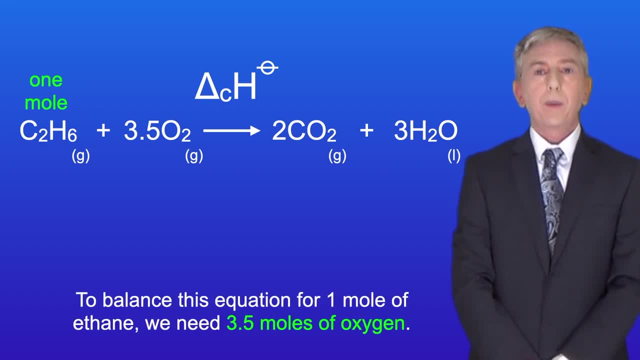 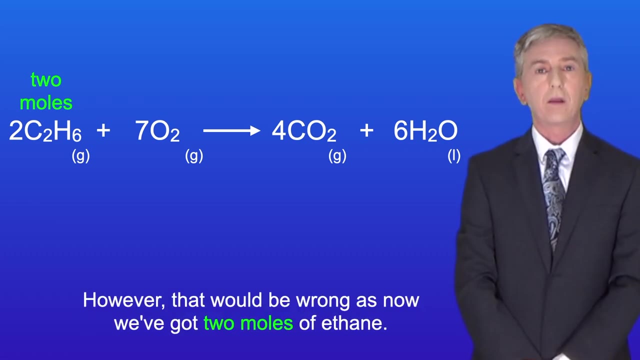 combusting one mole of ethane. To balance this equation, for one mole of ethane we need 3.5 moles of oxygen. Now it might be tempting for you to double everything, to make this a whole number like this. However, that would be wrong, as now we've got two moles of ethane. 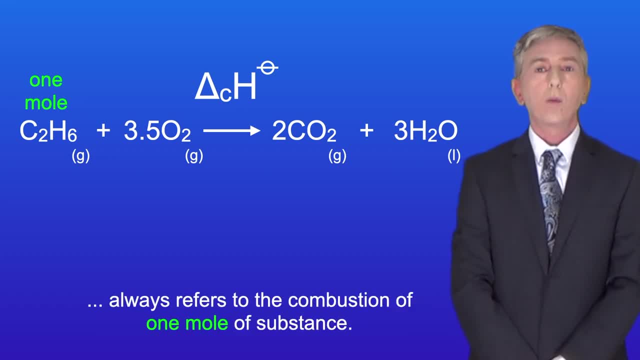 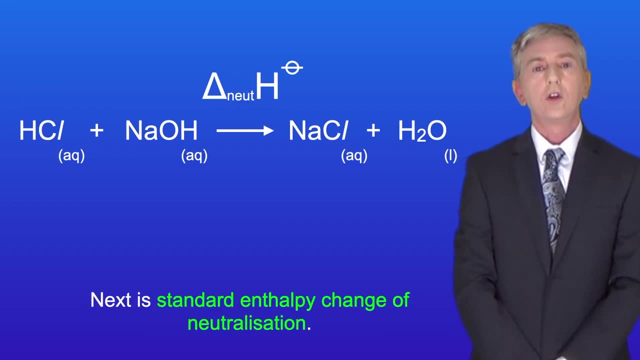 So you need to remember that standard enthalpy change of combustion always refers to the combustion of one mole of substance. Okay, next is standard enthalpy change of neutralisation. This is the enthalpy change when one mole of water is formed in a neutralisation reaction under standard conditions. I'm 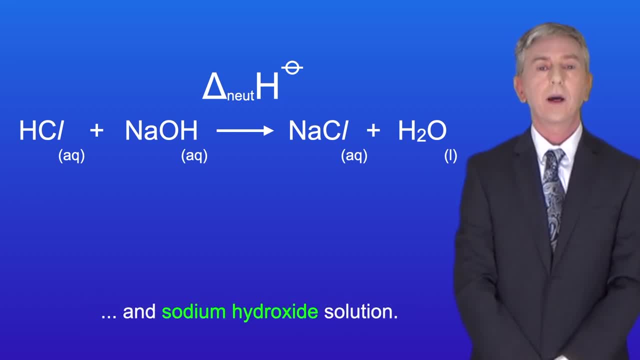 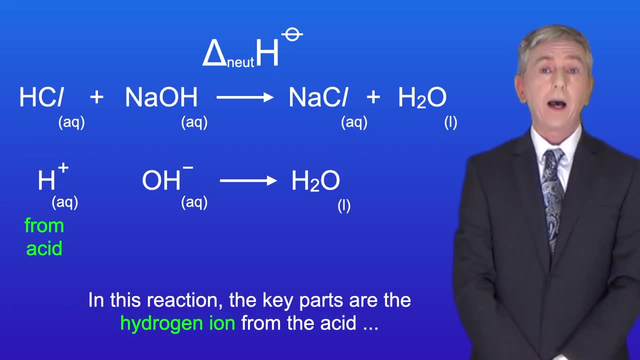 showing you the equation for this reaction here with hydrochloric acid and sodium hydroxide solution. Now, there is an interesting point about this. In this reaction, the key parts are the hydrogen ion from the acid and the hydroxide ion from the alkali. So what that? 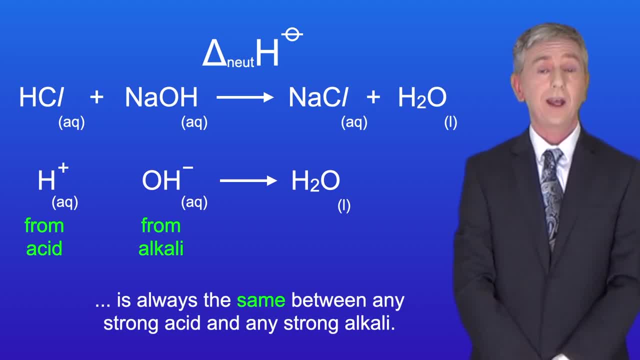 means is that the standard enthalpy change of neutralisation is always the same between any strong acid and any strong alkali, and this value is minus 57 kilojoules per mole. As you can see, this reaction is exothermic and we're going to look at how to determine. 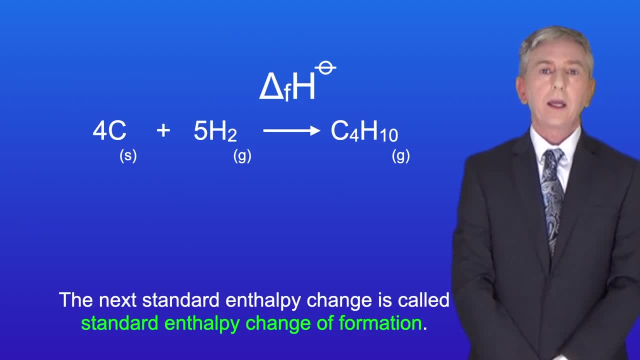 this enthalpy change in a later video. Okay, the next standard enthalpy change is called standard enthalpy change of formation. The standard enthalpy change of formation is the enthalpy change when one mole of a compound is formed from its elements under standard conditions and all of the chemicals. 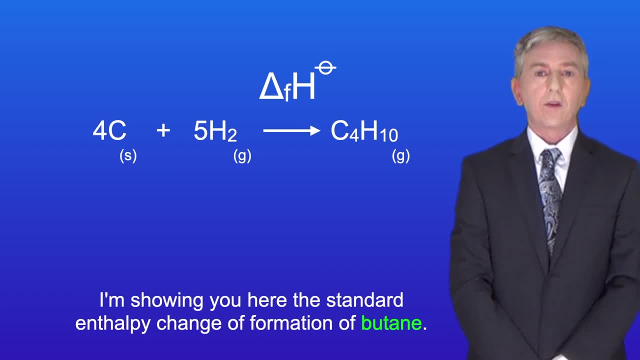 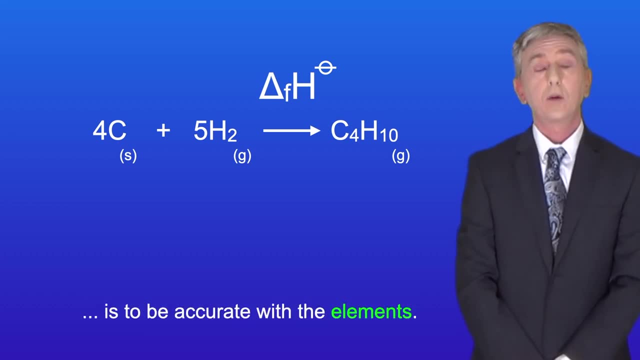 are in their standard states. I'm showing you here the standard enthalpy change of formation of butane. Now, the key thing with standard enthalpy change of formation is to be accurate with the elements. As you can see, we're reacting 4 moles of carbon with 5 moles of hydrogen. 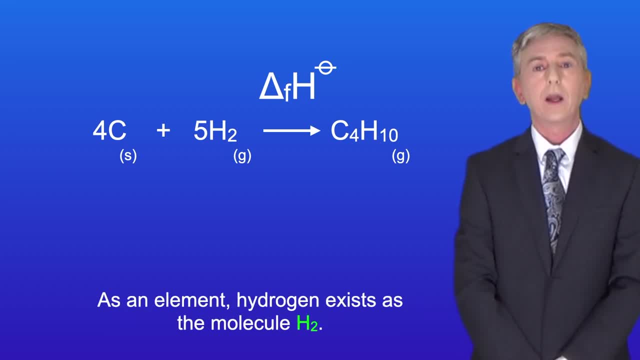 Now as an element. hydrogen is the element that is formed from the elements, So the hydrogen exists as the molecule H2.. Some students forget this and write hydrogen as simply H, which is wrong. So always double check that the elements are accurate And 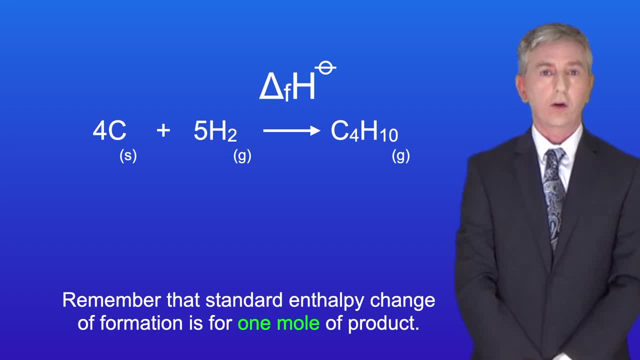 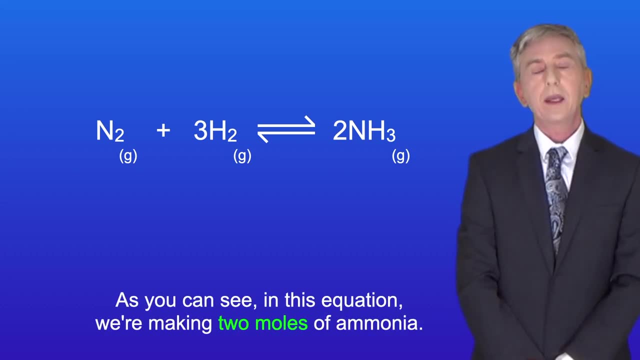 remember that standard enthalpy change of formation is for 1 mole of product. I'm showing you here the equation for the formation of ammonia. As you can see, in this equation we're making 2 moles of ammonia. So for standard enthalpy change of formation.